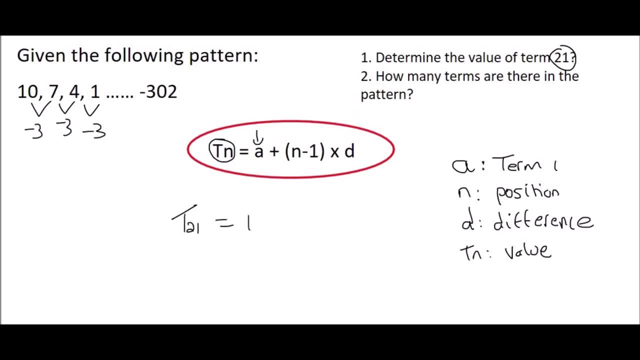 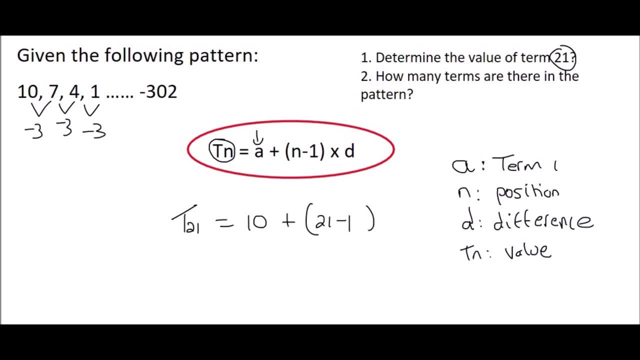 for is 21.. So we say 21 minus 1, and then the difference is negative 3.. Just remember, guys, that's negative 3, not positive 3.. Then you simply go and work this all out on the calculator if you and you end up with minus 50.. So what that means is that if we had to carry on with this pattern, 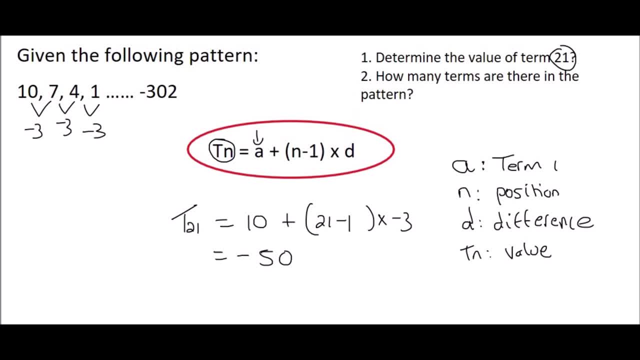 until we get to the 21st term, the number that we would see there would be negative 50.. The next question says how many terms are there in the pattern. So we could go from 10 all the way to minus 302 and we could write those numbers down. 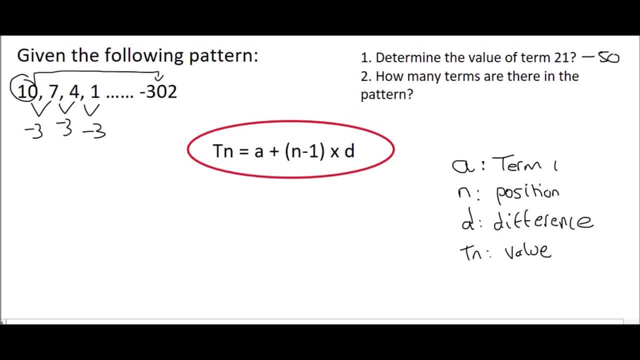 and it would probably take three or four pages of writing, but you would still get there. but then remember there's a faster way. So we need to look at that minus 302 and ask ourselves: is that the position or is that the actual value at that place in the sequence? So is that going to be a tn? 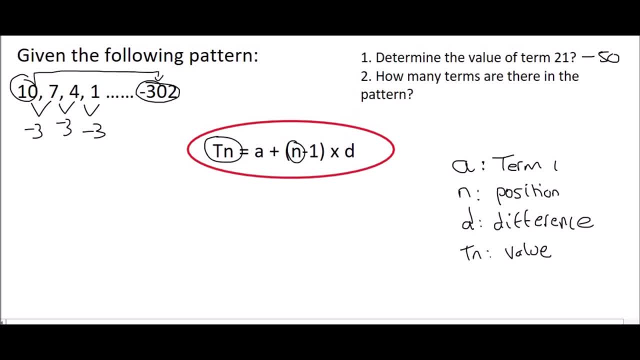 or is that going to be a n? Well, well done to you. if you say tn, that is actually the. that is the value that at that point. So we will substitute that in the front of the equation. a is 10, we don't know n, because we don't know which position that would be, and then the difference is negative. 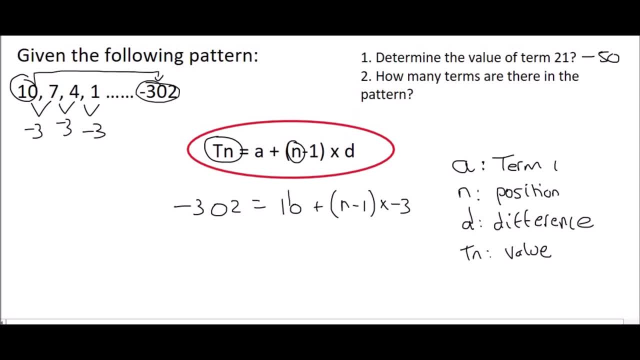 302. Now solving, and there are multiple ways to do this, but I'm going to take the 10 over then, this times by minus 3.. I've seen many issues in my past with students who battle with this, so if you are going to multiply it into the bracket, please remember that it goes to the n and it goes to the 1, okay, 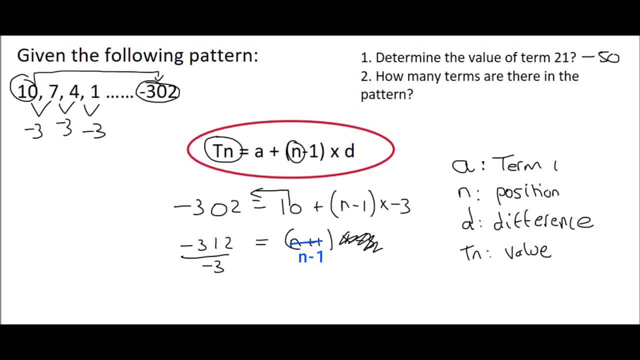 but the other option is 104, because the negatives would cancel, and so you're left with 104 equals to n plus 1, and so n is 104.. So what that means is that if you had to keep going in the sequence after you have gone, well, 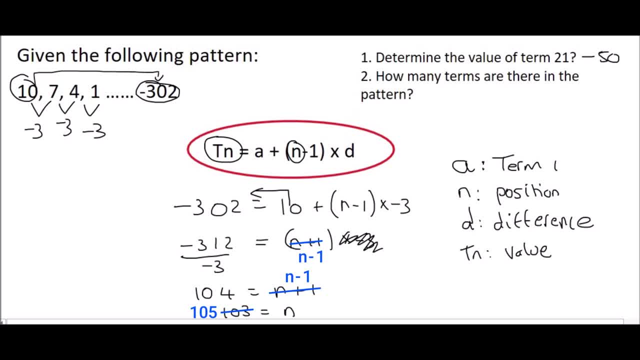 once you arrive at the 103rd position, the value that you would see there is negative 302..